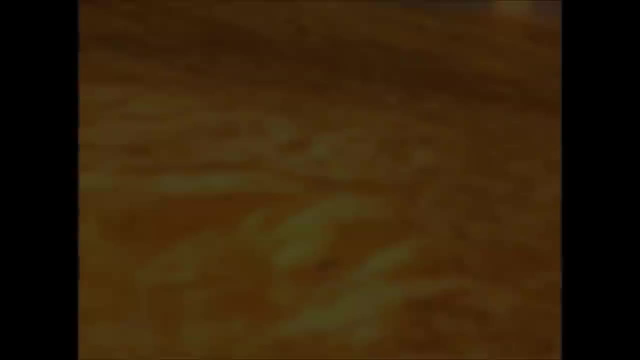 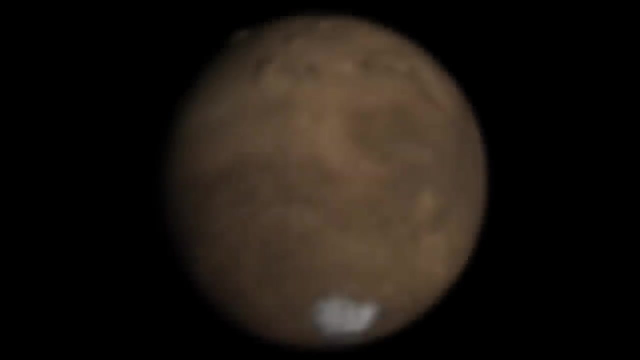 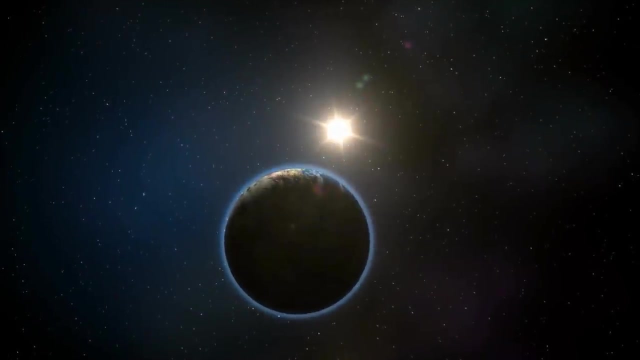 that has liquid water on its surface. Other planets are either too hot, causing all their water to evaporate into gases, or too cold, causing any water they have to freeze into ice. The Earth is about 93 million miles or 150 million kilometers away from the Sun, which 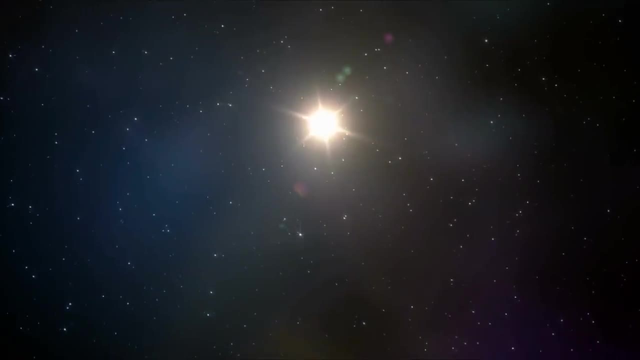 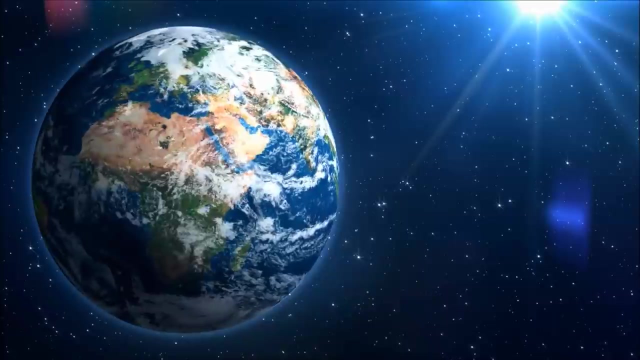 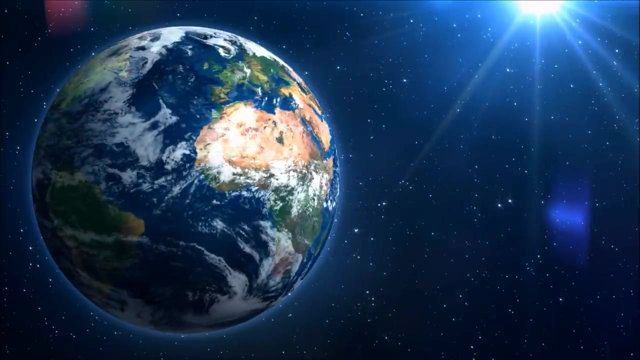 keeps it at just the right temperature to have liquid water. And the Earth has a lot of water. More than 70% of the Earth's surface is covered by oceans. That means that the oceans are more than twice the size of all the land on Earth. Because Earth has so much water? 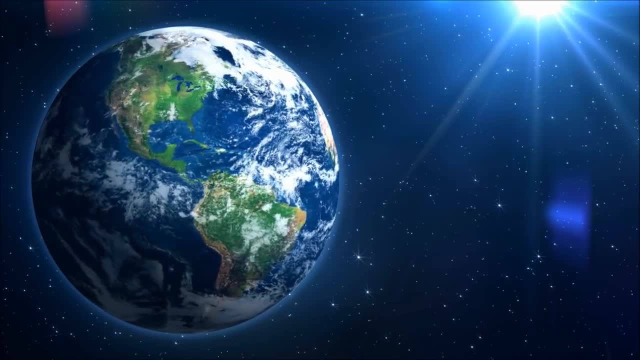 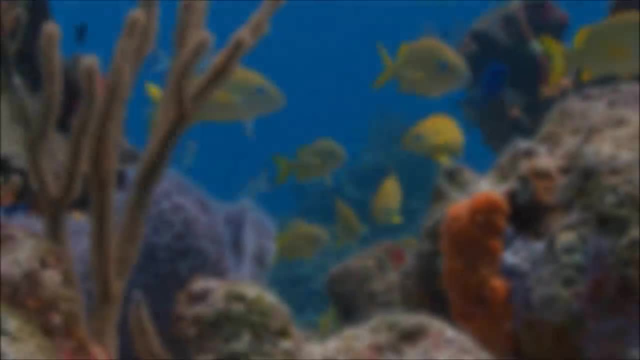 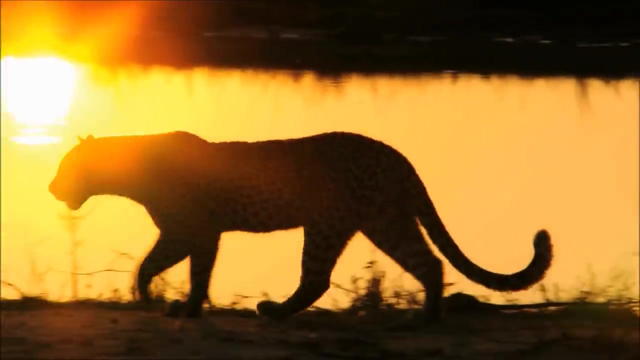 on it. it is sometimes called the Blue Planet. Liquid water is what allows life to exist on Earth. As far as we know, Earth is the only place that life exists. Millions of species of plants and animals call the planet Earth home, including humans. 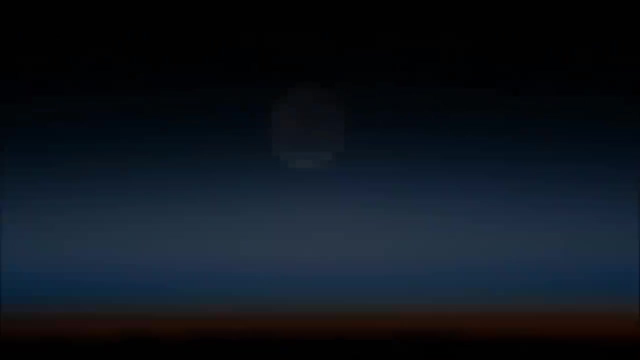 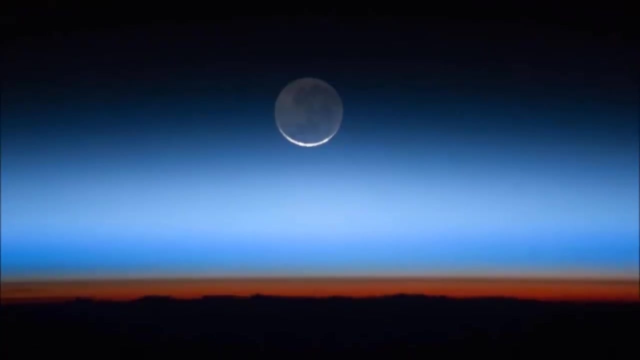 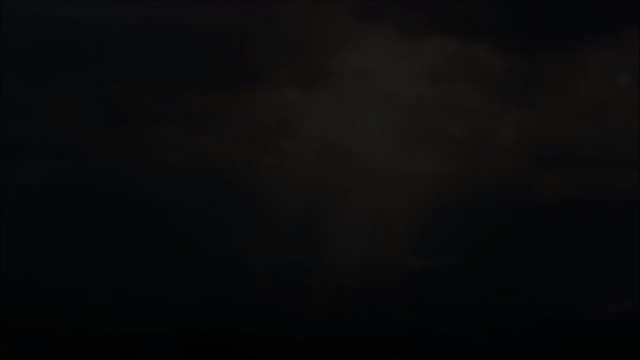 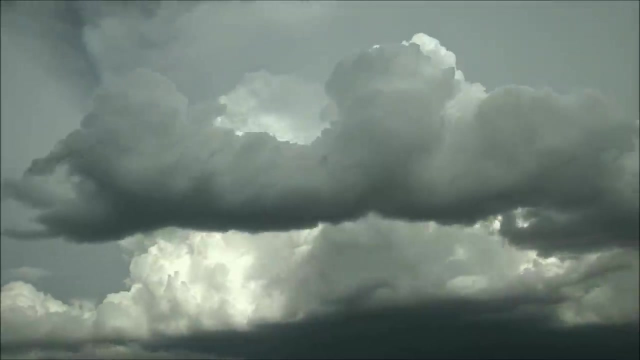 Earth's atmosphere is another important feature. The atmosphere is a thick layer of gases that covers the entire Earth. It is mostly made of nitrogen and oxygen. The atmosphere is what allows us to breathe. It also helps keep the Earth warm by acting like a blanket to hold in the sun's heat. 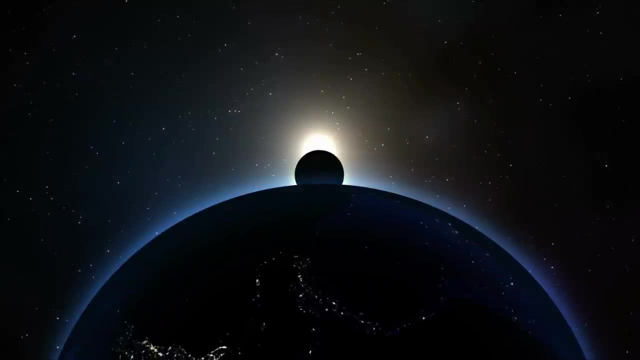 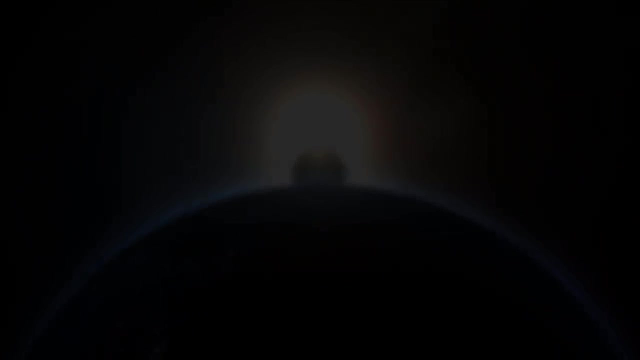 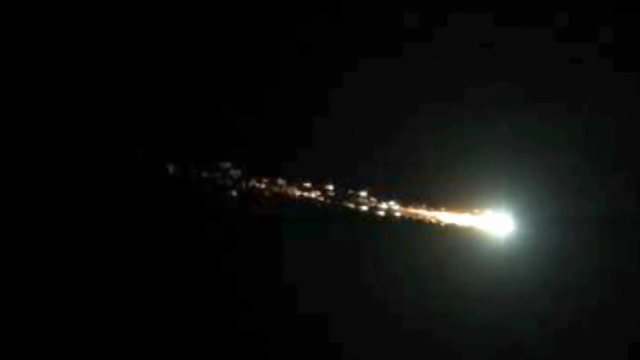 Another way the atmosphere helps us is by protecting the Earth from harmful radiation from the sun and also from meteors. Anything falling to the Earth from space is rubbed against the gases in the atmosphere until they burn. Most things burn up completely before they reach the surface, but even anything that 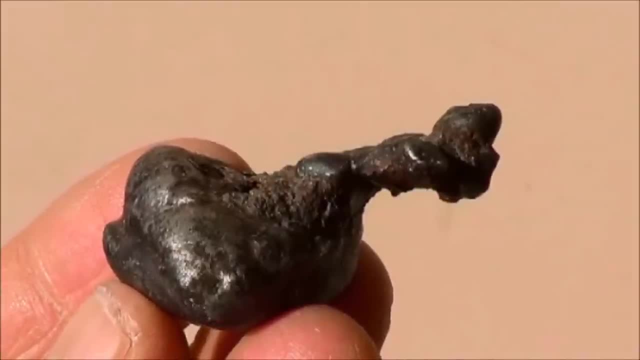 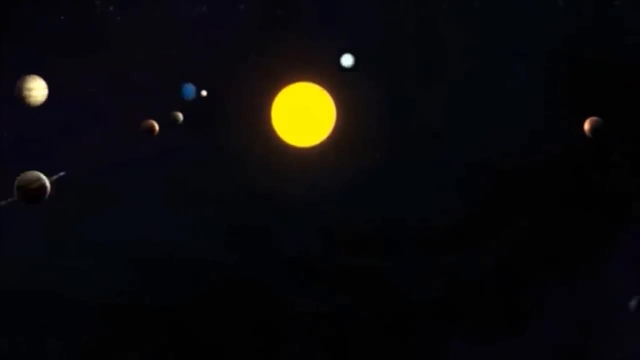 makes it through is much smaller by the time it hits the ground. The Earth goes around the sun. The time it takes to go around the sun is called a year. It takes the Earth about 365 days to travel around the sun once. That is why a year is usually 365 days. 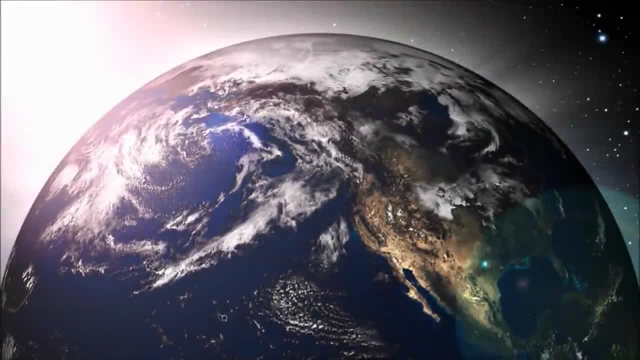 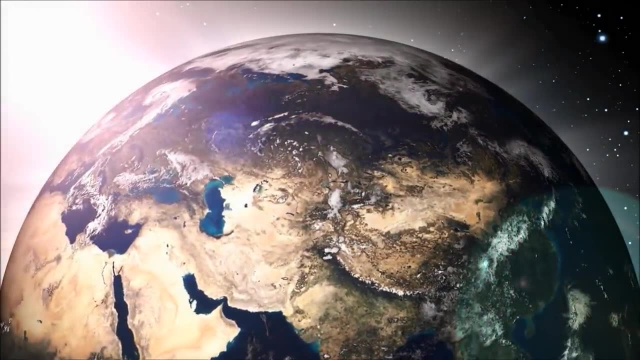 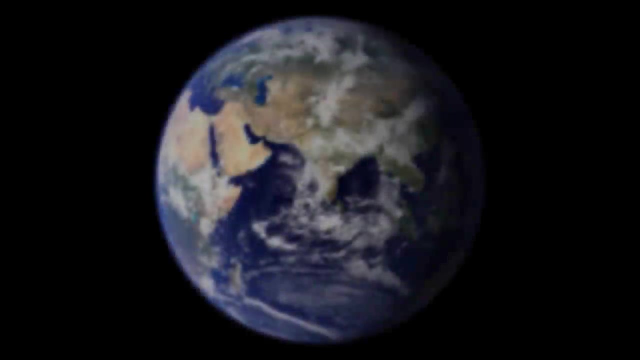 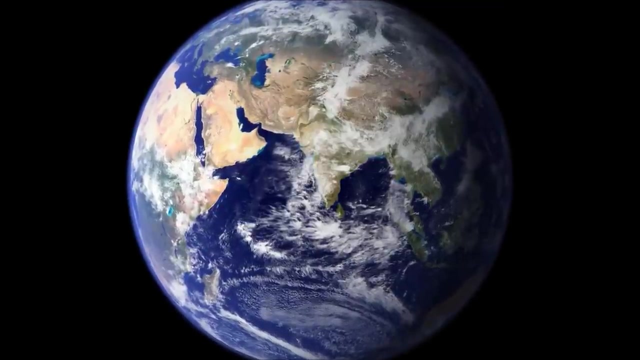 The Earth also rotates, or spins. The time it takes for the Earth to rotate once is called a day. The Earth rotates every 24 hours and that is why a day is 24 hours long. The Earth does not rotate straight up and down. 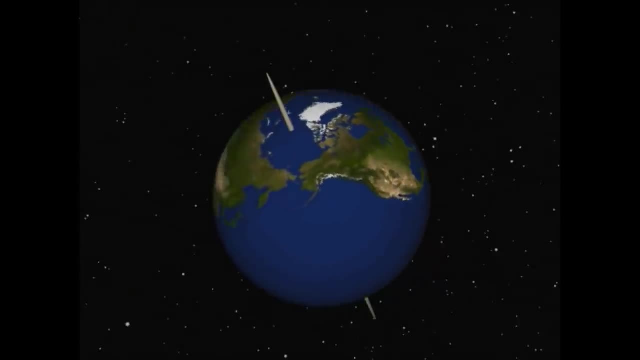 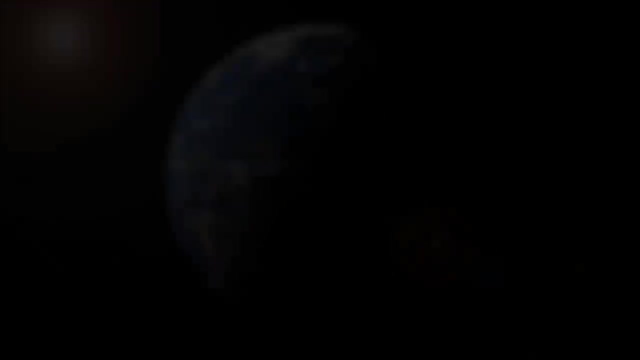 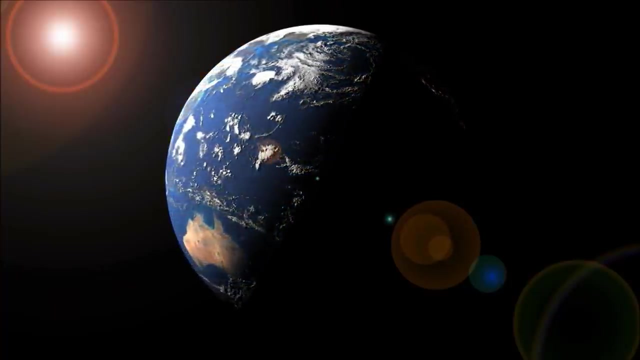 It is tilted. There is an imaginary line through the Earth, from the North Pole to the South Pole, called the Earth's axis, and this axis is tilted at about 23 degrees. Why is it important that the Earth is tilted? Well, the tilt of the Earth's axis is what causes the seasons. 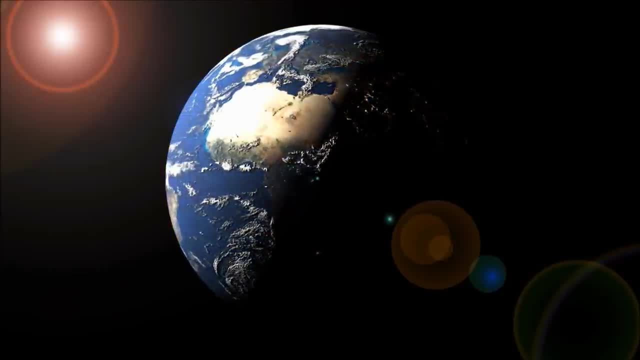 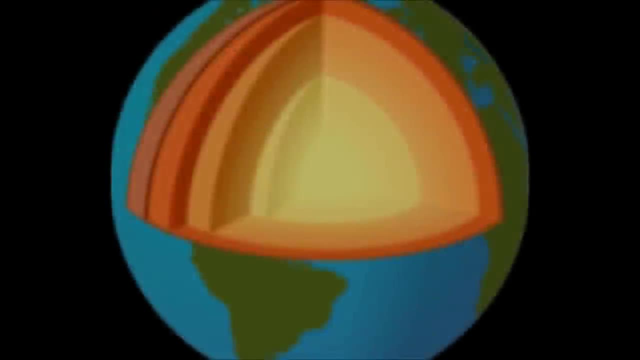 When a part of the Earth is tilted towards the sun, it will be summer. there, The Earth is tilted. The Earth is tilted. When it is tilted away from the sun, it will be winter instead. The inside of the Earth is very different from the outside. 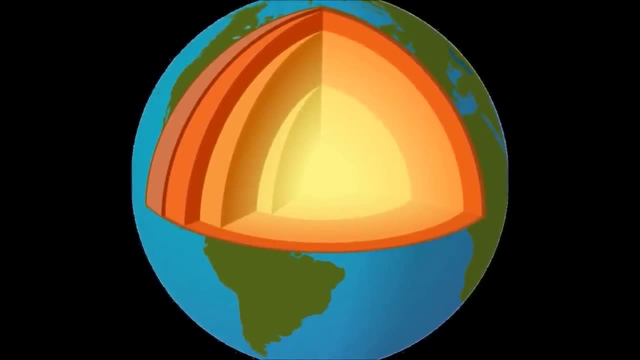 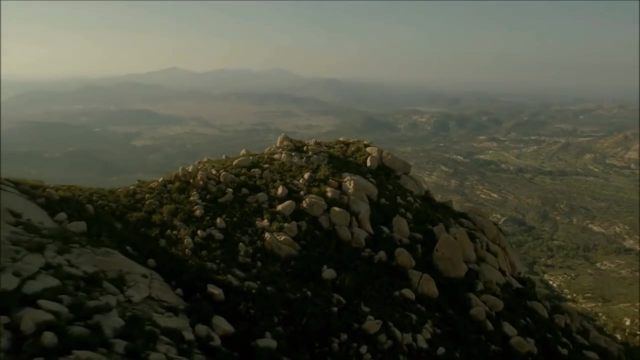 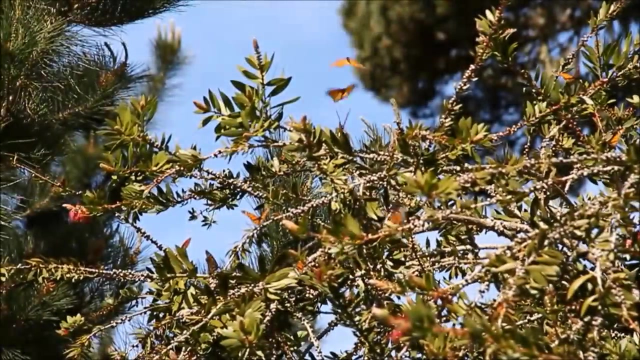 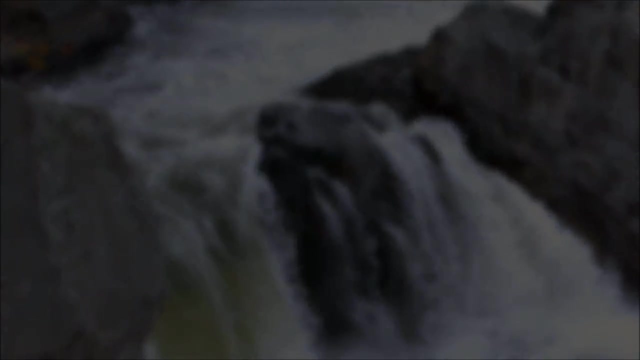 If you were to cut the Earth in half, you could see that it is made up of different layers. The outermost layer, called the crust, is where we live. The Earth's crust is cool and solid. Everything you see- trees, mountains, rivers, houses and even the oceans- are sitting on. 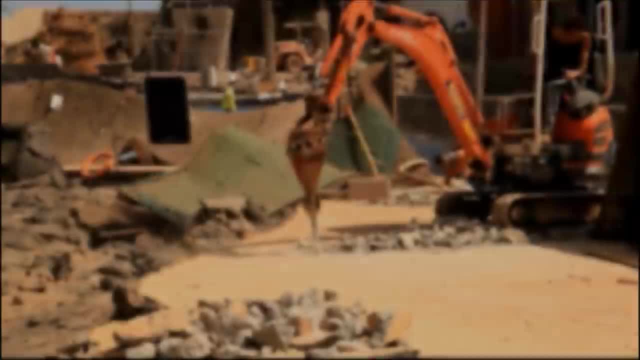 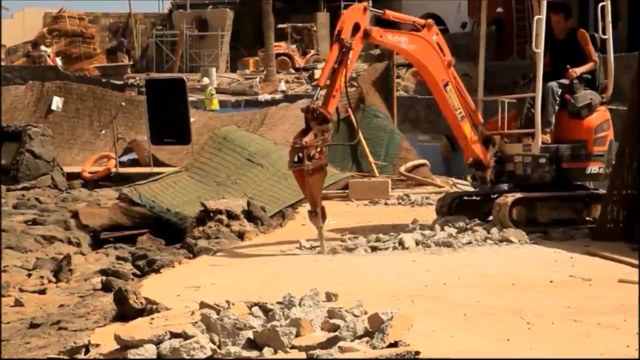 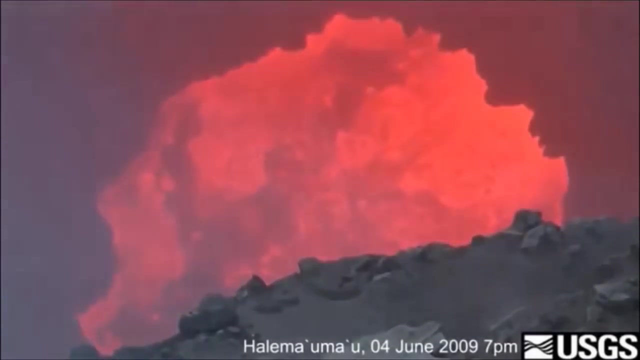 top of the Earth's crust. The crust is so thick that humans have never been able to dig deep enough to break through it. But the crust is only a thin layer on the surface of the Earth. Underneath the crust is the mantle. The mantle is a thick layer of molten rock or magma. 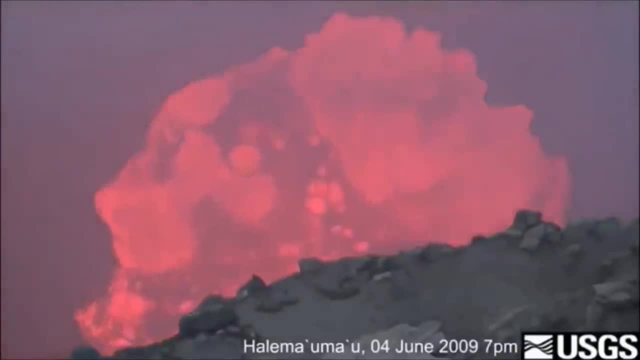 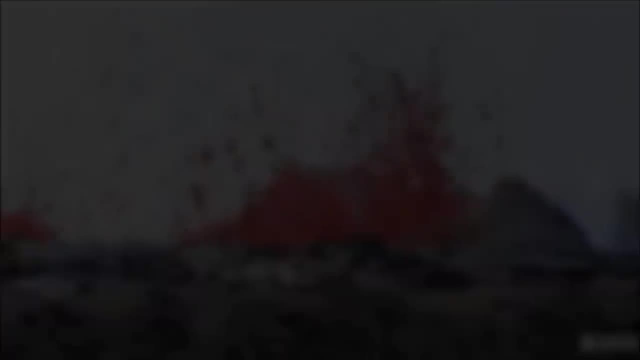 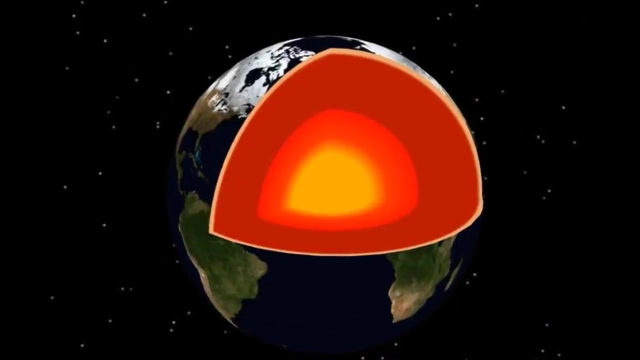 It is the thickest layer of the Earth. Sometimes magma from the mantle will come up to the surface through volcanoes. The core is at the very center of the Earth and it is very, very hot, with a temperature of thousands of degrees.